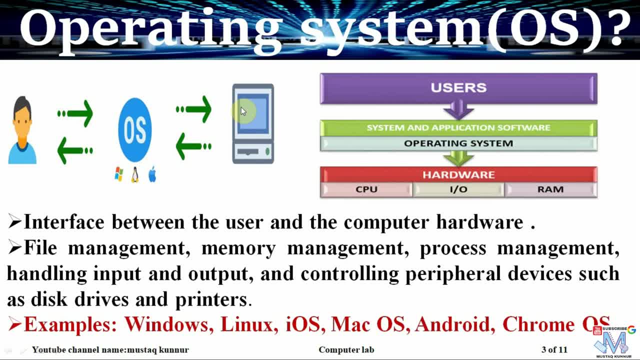 by a computer hardware. Once the computer hardware gets the command from the operating system, it processes it and sends the result to the user through operating system. In this way the operating system works as interface between the user and computer hardware. When we buy a new laptop, a computer or any cell phone, we must install the operating system. 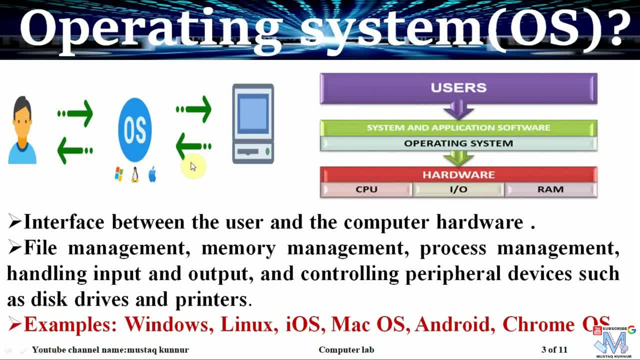 first. Without installing operating system we cannot run that device Here in this figure we can see that after installation of operating system we can install the application programs. Once we install the operating system and application program then user can communicate with the computer. hardware Operating system also has different functionalities. It is also used. 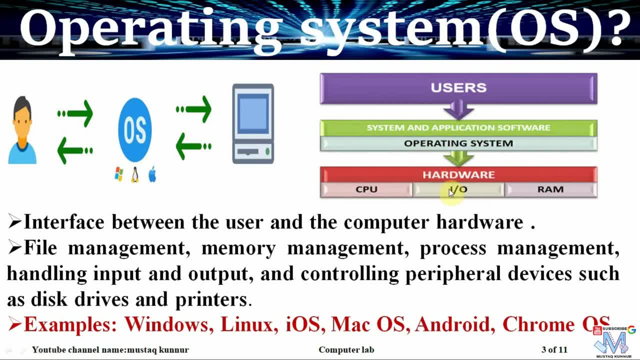 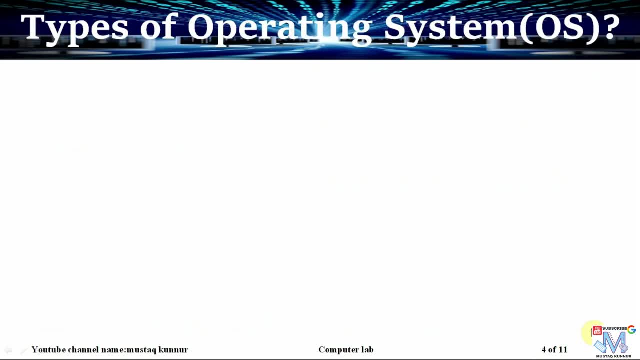 to manage the CPU and input output devices, and it is also used for the computer hardware. The few examples of operating systems are Windows, Linux, iOS, Mac OS, Android and Chrome OS. Now coming to the types of operating system, It is generally classified into five categories. 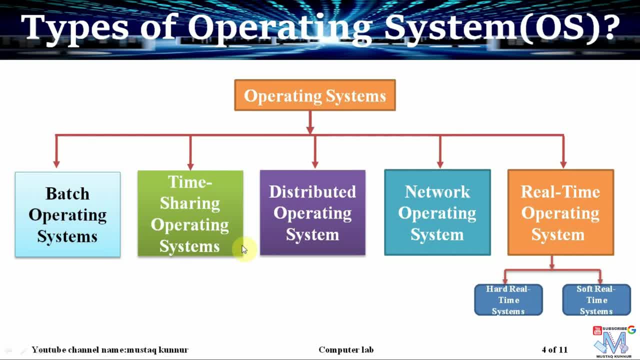 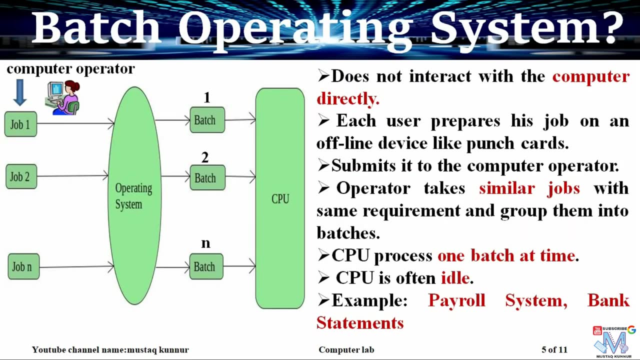 that is, batch operating system, time-sharing operating system, distributed operating system, network operating system and real-time operating system, also known as RTOS. This system is further classified into two categories, that is, hard real-time system and soft real-time system. In batch operating system- here user does not interact directly with the computer. 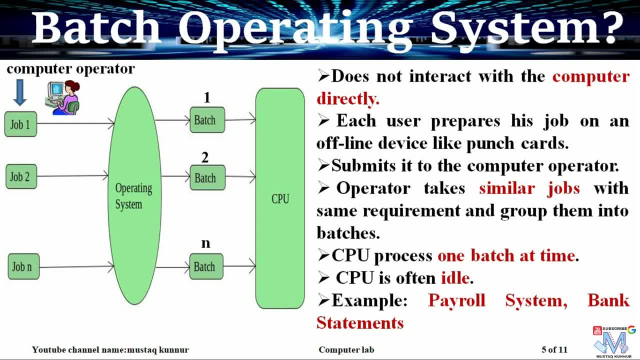 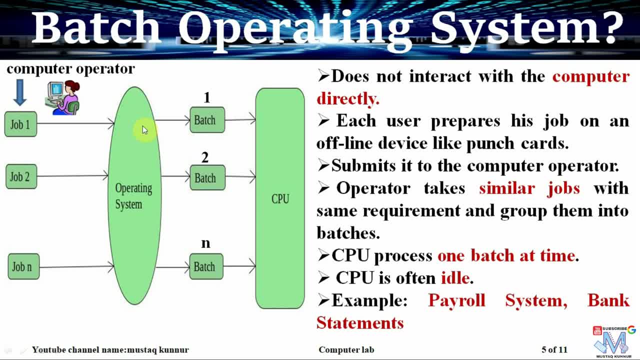 Then operating system send that group of job or batch of job one after another to the CPU. CPU is a central processing unit. In this figure we can see that initially it takes batch 1. Once the batch 1 is completely processed, then it goes to batch 2. 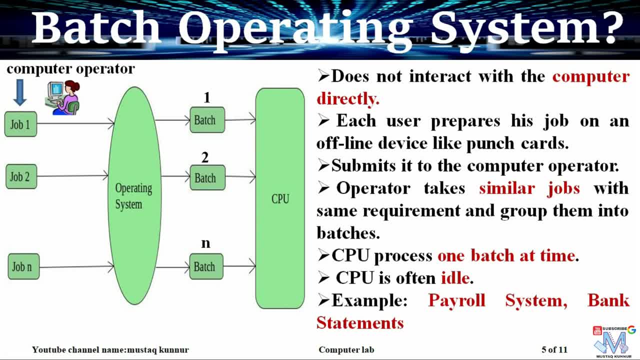 Similarly, it process all the batches. In this type of system, the batch operating systems are used. In batch operating system we can see that CPU is usually idle while switching from one batch to another batch. This is the disadvantage of the batch operating system. The few example of batch operating systems are: 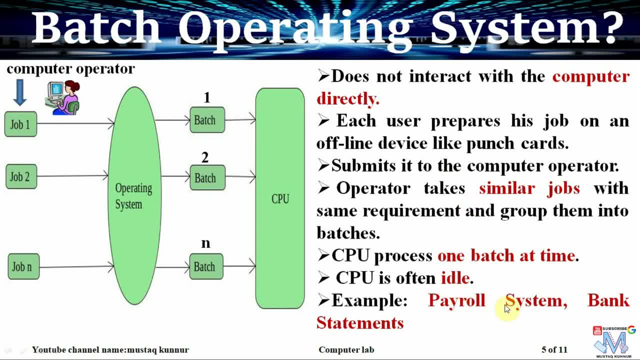 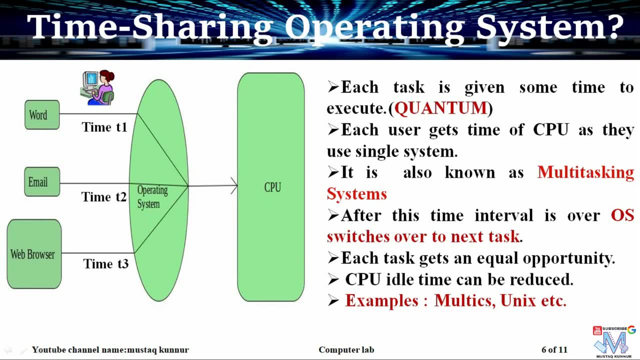 The operating system which are used in payroll systems in order to generate the salary bills. Similarly, the operating system which is used to generate the bank statements In time sharing operating system. we can see that here The user is operating system Operating on multiple tasks at same time, As in that a user is operating on word and email. 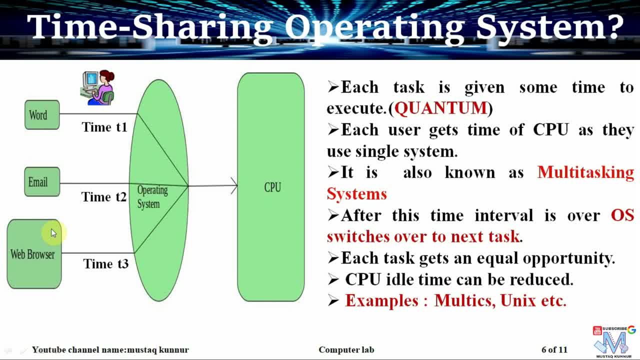 And he is also downloading some files from web browser And these three applications simultaneously operating on an operating system. Then operating system combine these three tasks and fed to the CPU. CPU process this, all the tasks at same time. How it process it, It takes the task one after another. 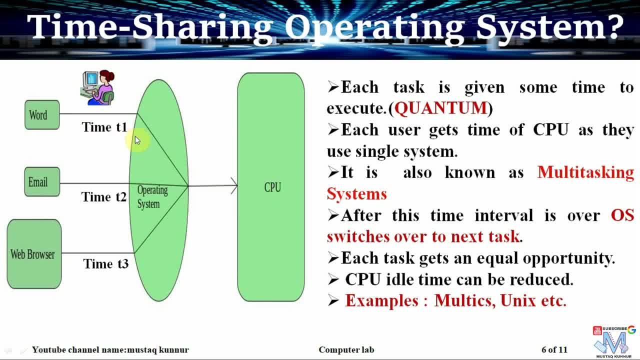 The CPU first assign some time to the word, that is time T1. It assigns some time to the email, that is time T2. It also assigns some time to web browser for downloading some files, that is time T3. First it finishes the task T1, Then switch over to task 2, that is email. 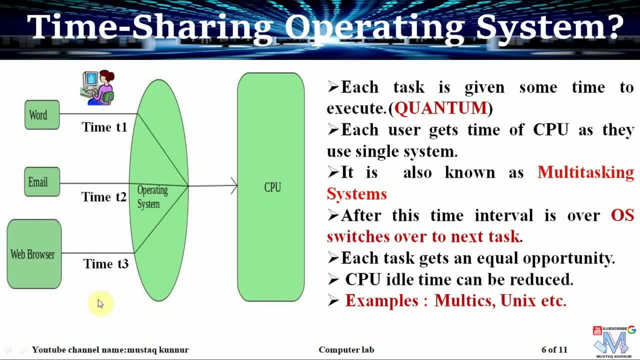 After completion of this task it switch over to next task, That is, downloading of file from web browser. It takes the time T3. The operating system is also assigned some time to the email. that is time. T1- amount of time assigned or taken by a CPU to complete a task is known as quantum. 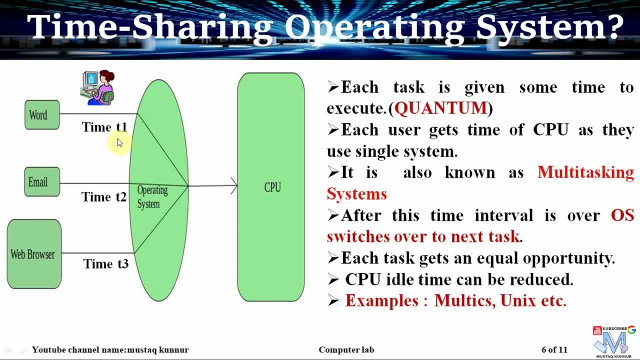 We can see that actually the CPU is processing each task sequentially one after another. Since the switching time is in terms of microsecond, the user gets feel of multitasking. In this time-sharing operating system, the CPU idle time is substantially reduced. Few examples of time-sharing operating systems are Multics, Unix. 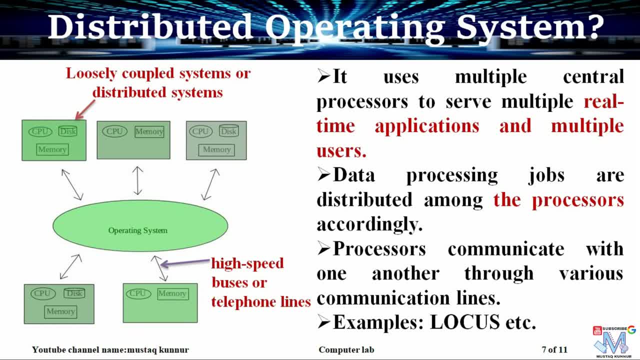 Now coming to the distributed operating system. Distributed operating system usually uses multiple processors. In this figure we can see that we have multiple processors or multiple CPUs. These are connected together with the help of multiple processors, This type of high-speed buses or telephone lines. 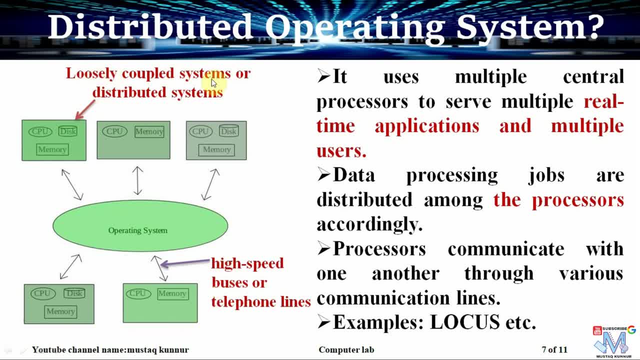 These type of systems is also known as loosely coupled systems, because the one CPU does not have sufficient information about another CPU. Hence it is called loosely coupled system. In this figure we can see that when a task is assigned to this computer, then this computer 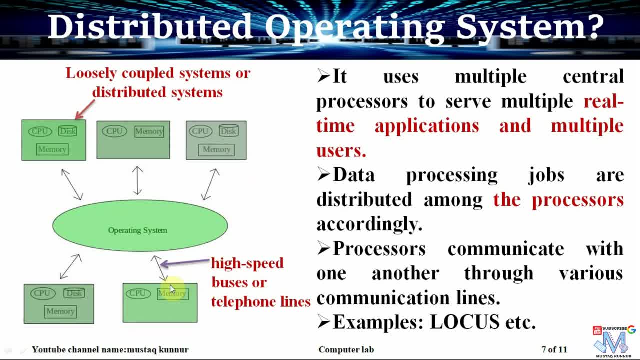 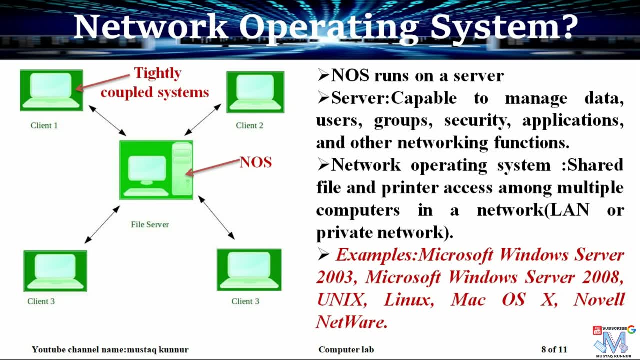 distributes the task among all the processors, Hence it processes the task with very high speed. The example of distributed operating system is locus. Now coming to the network operating system, We know that network is a group of the computer. The network may consist of server as well as client. 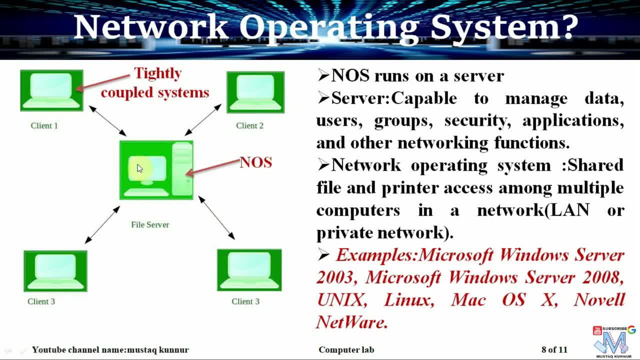 Usually the network operating system is installed or reside on the server. We know that server is a computer which is capable of managing the data and users and resources, All the clients usually connected to the server, And the operating system is distributed. The operating system which resides at the server is used to share the files, share. 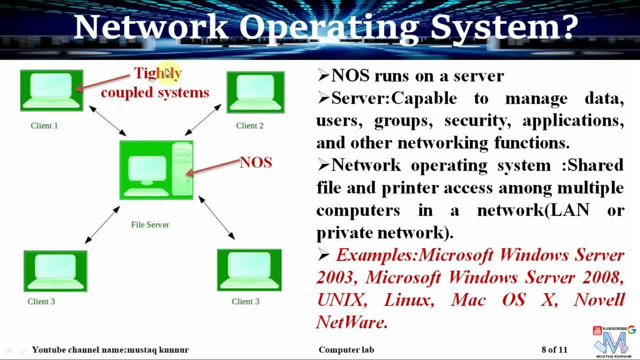 the resources. Hence we can say that network operating system is used in the server. The few examples of network operating systems are Microsoft Windows Server 2003,. Microsoft Windows Server 2008,, Unix, Linux, Mac OS X, Novel Network. Now coming to the real-time operating system. 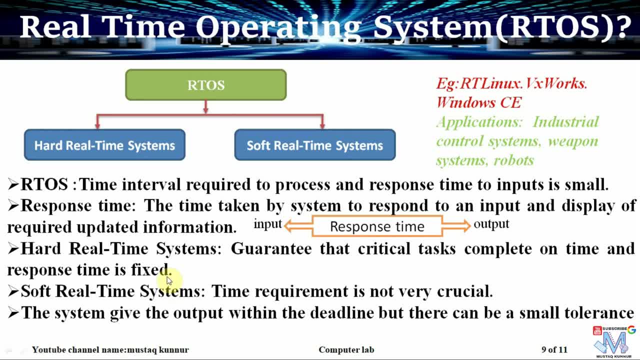 That is also known as RTOS. RTOS. it is used for real-time application. Its response time and process time is very small. What is response time? Response time is time taken by a system to get the input and to give the output. 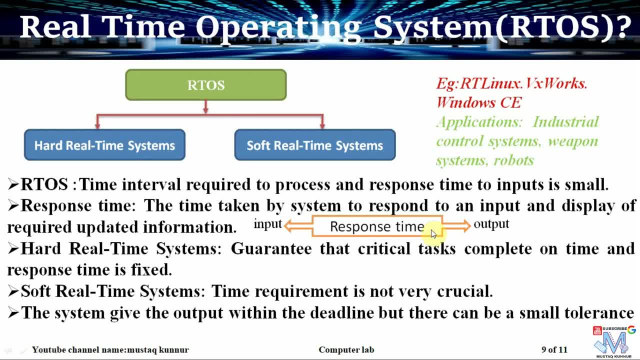 That is known as response time. In RTOS the response time is very small. RTOS can also be classified into two categories, That is, hard real-time, Hard real-time system and soft real-time system. In hard real-time system, the response time is fixed. 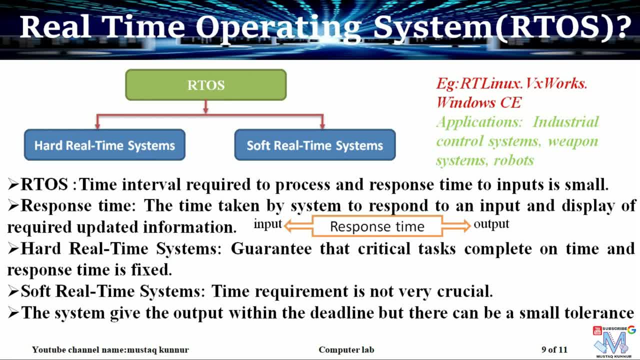 Whereas in soft real-time system the response time is not fixed. It has some tolerance, but it has some deadlines. Within a deadline it must process its task. The few examples of RTOS are RT, Linux, VxWorks, Windows CE. 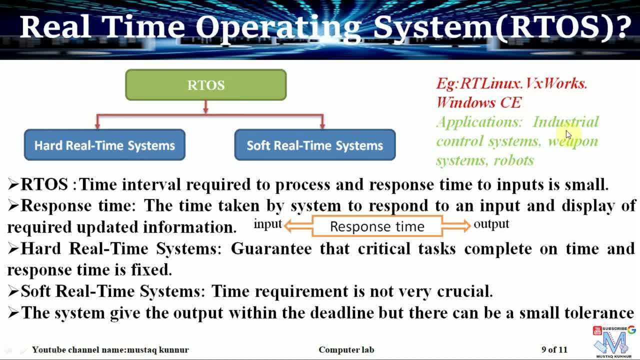 These type of RTOS are used in the software. In the software the response time is fixed. They are used in the applications like industrial control system, weapon system and robots. These type of RTOS are also used in the embedded systems and the critical applications like 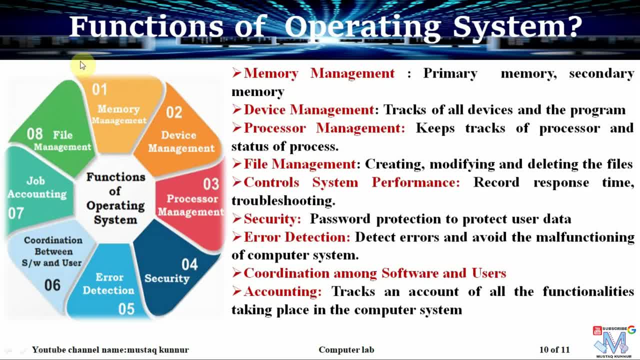 satellite. Now coming to the functions of operating system, Operating system facilitate these following facilities. Number one is memory management. The OS is used for the memory management of primary memory as well as secondary memory. We know that RAM is a primary memory. 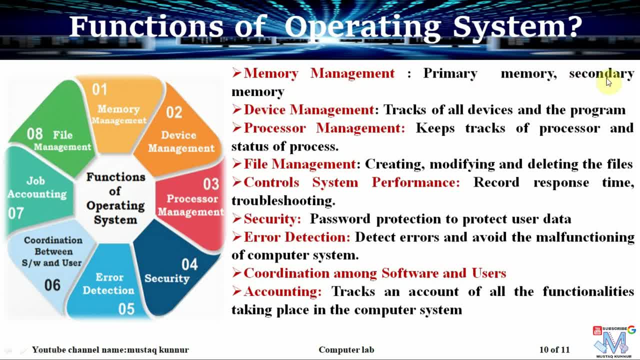 Hard disk is a secondary memory. In order to manage these two memory, operating system is needed. It is also used for the device management, That is, in order to track the programs and functions of all the devices which is connected to the computer, the operating system is needed. 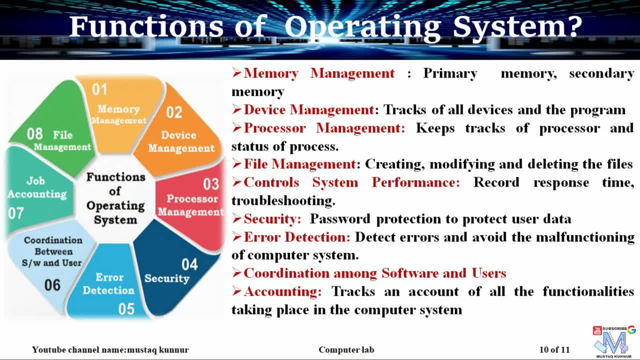 Similarly, in order to keep track of the processor and the status of process, the operating system is needed That is called process management. In case of creating the files, modifying the files and deleting the files, we need operating system That is called file management. 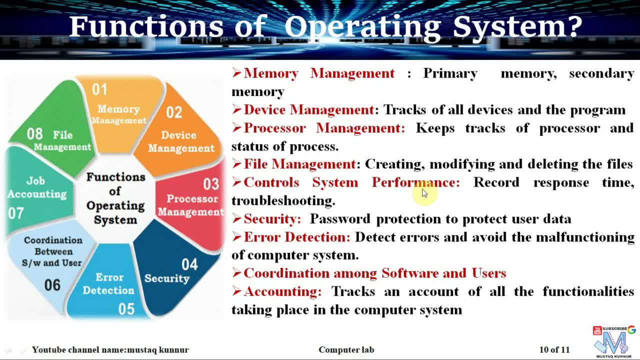 Whereas control system performance, It records the response time, and it is also used to troubleshoot an application That is called control system performance. As far as security is concerned, in order to protect our computer or any application, the password protection is required, and that is provided by the operating system.